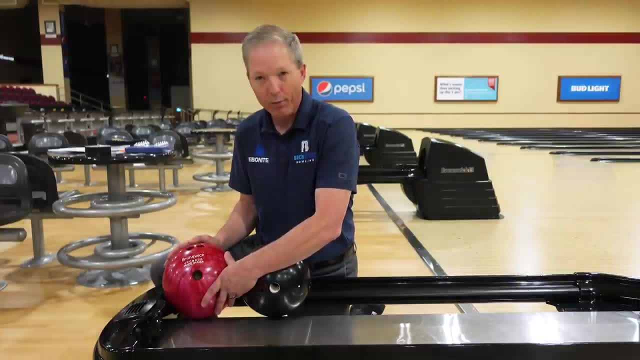 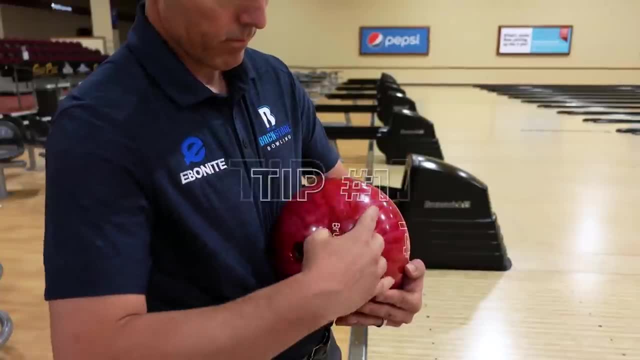 this is what you're going to see at the bowling center. These are low performance bowling balls. They're very durable. You put your whole hand, your fingers, your thumb, all the way into the bowling ball. The grip really doesn't fit you and they go from point A to point B on a very 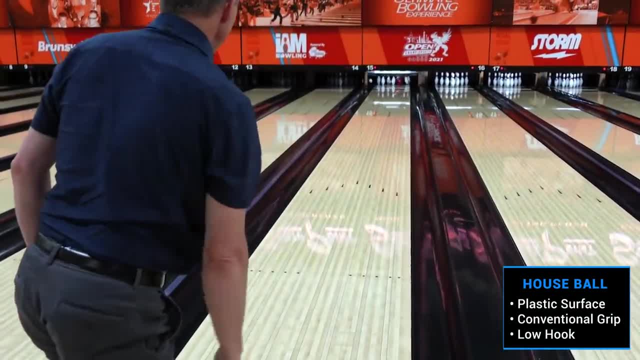 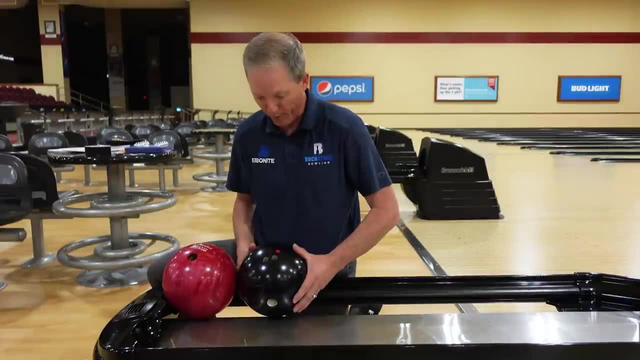 straight line. It's very difficult to knock down pins when you can't get the ball to hook, And the other ball that we want you to go look at and see a local certified pro shop operator is a high performance ball. This ball the outside. 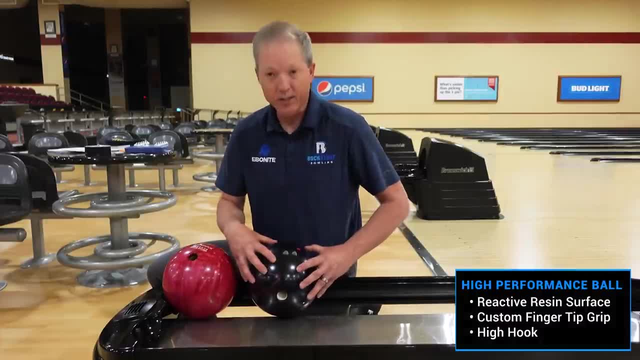 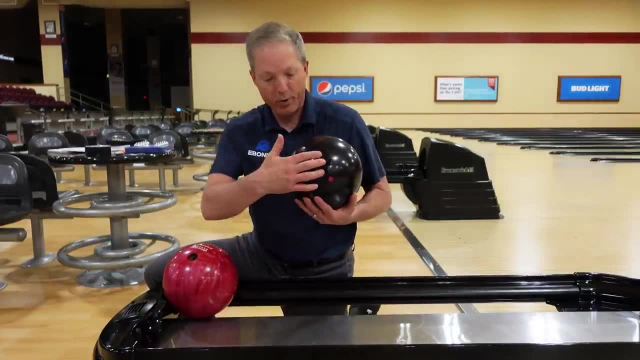 it does have characteristics for the ball to hook. The inside's much different. There's a lot of physics. The core structure is very dynamic: Your grip- we call this a fingertip grip- Just the ends of your fingers. the first joint goes in, thumb goes all the way in. It's very secure. 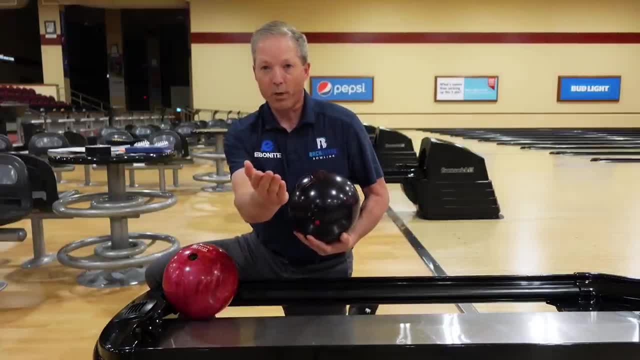 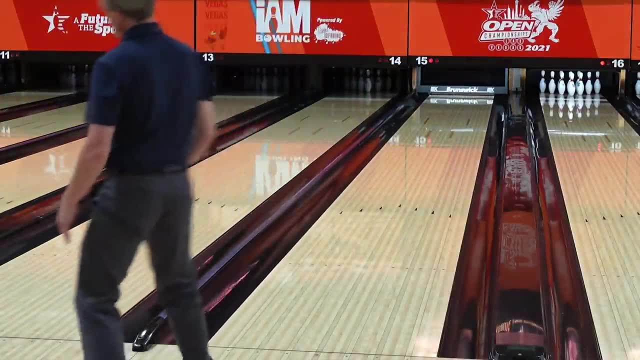 Your thumb's going to come out. You're going to be able to spin the ball. Now we're going to get the ball to hook, which is very important for you to increase your pins on your score. So we have two very different bowling balls. Beginner, this is a high performance. 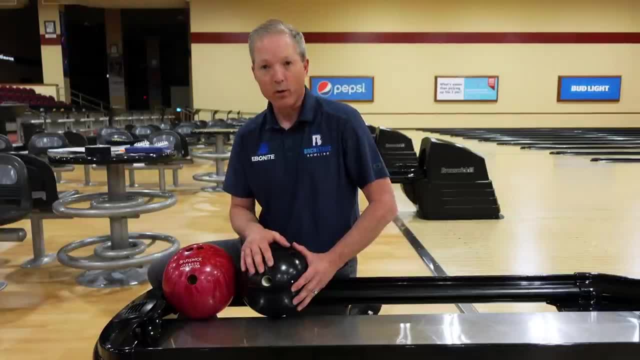 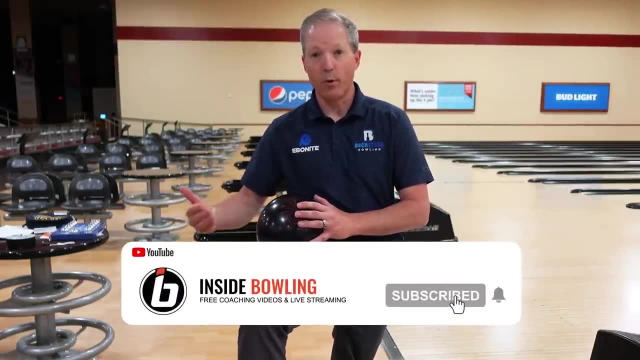 This is the one. you got to go see your local pro shop operator and go purchase. So we chose number one, the bowling ball. The second thing, and it's very underrated, is coaching and sport of bowling. Hey, we are just like any other sport. You've got to go see a certified coach who knows. 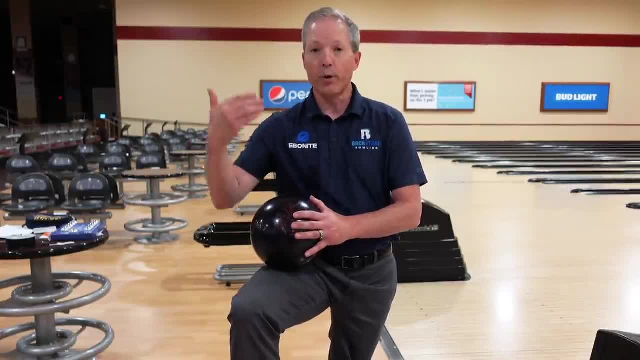 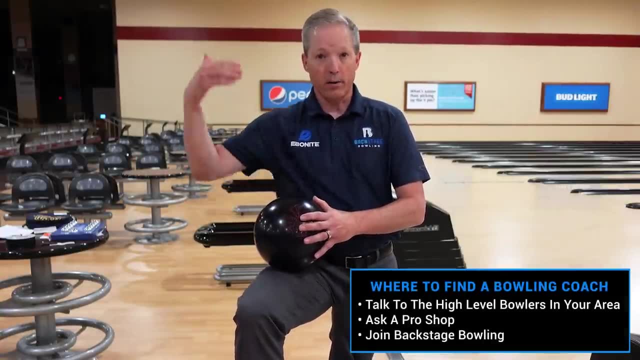 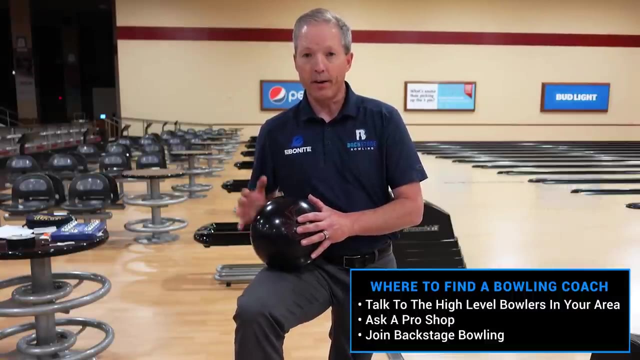 the game so we can put you from the start to the finish and really start developing those skills So important. Where do you find that coach? I would recommend go see some of your local higher level coaches. If you can't, we've actually got a link at the end of this video that you can get. 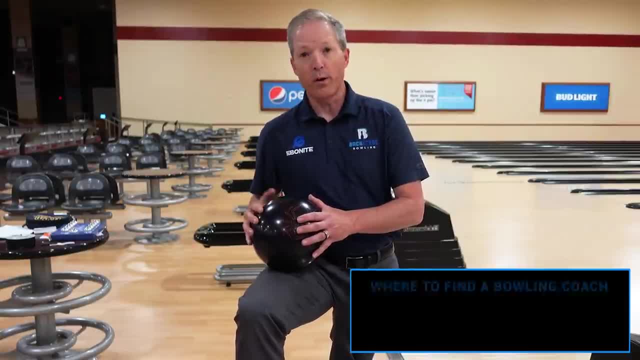 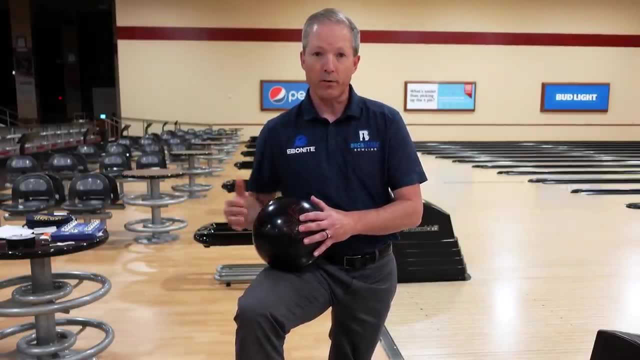 involved with and that'll actually help you as well. But, very important, you can see a coach. You got to get on a regular basis so you can develop those skills, so you can improve where you are right now to a competitive bowler. So we're going to talk about the third tip on going from a 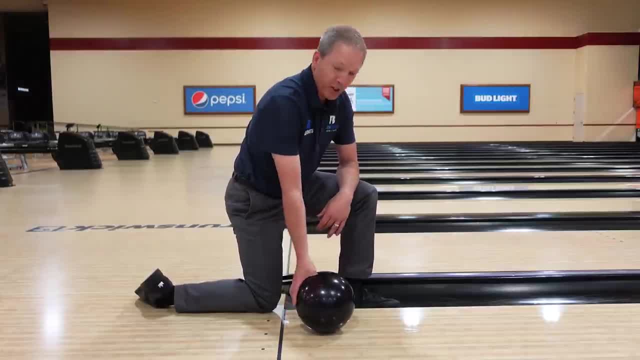 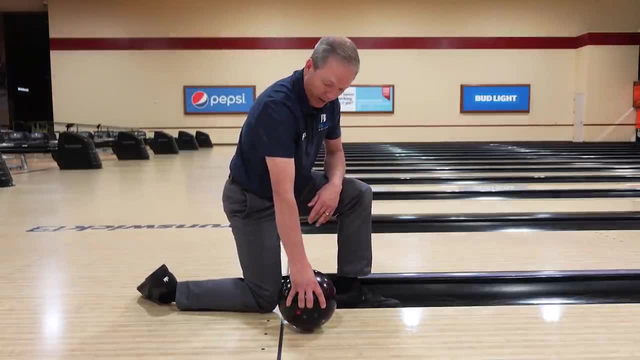 beginner to a competitive player. It's the release: getting the ball to spin off your hand. so we can get that spin off. Now we've got all the capability. Now we got to get our hands. so it's underneath to the center of the bowling ball. This is a great drill. Just put your left foot for right handers.